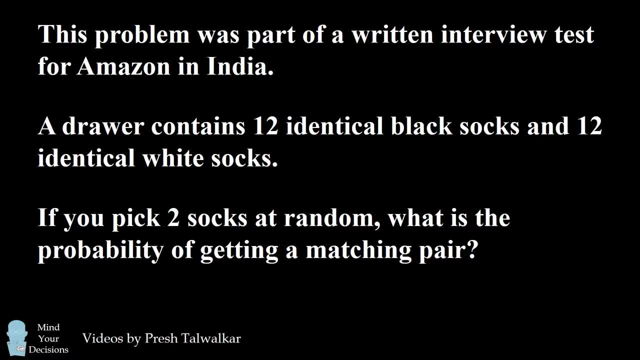 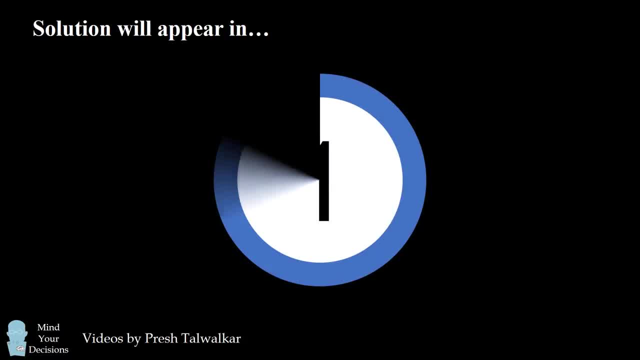 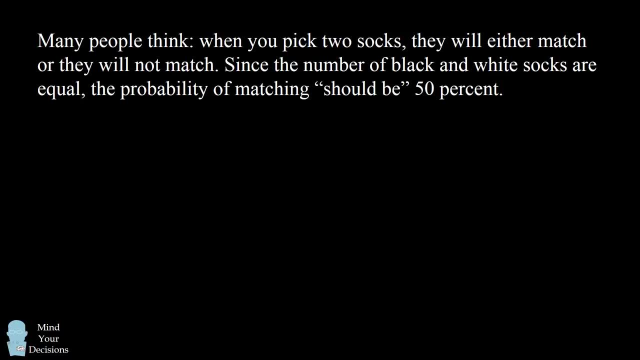 Can you figure it out? Give this problem a try and, when you're ready, keep watching the video for the solution. Many people think when you pick two socks, they will either match or they will not match. Since the number of black and white socks are equal, the probability of matching should be 50%. 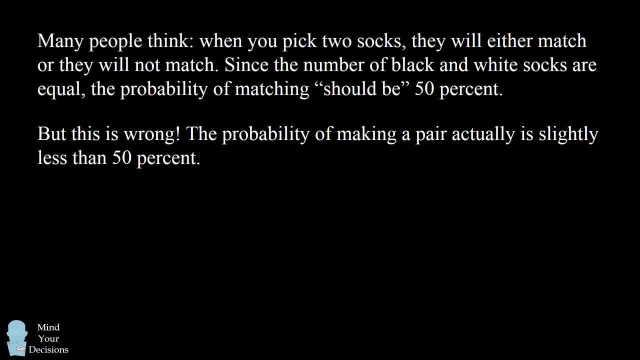 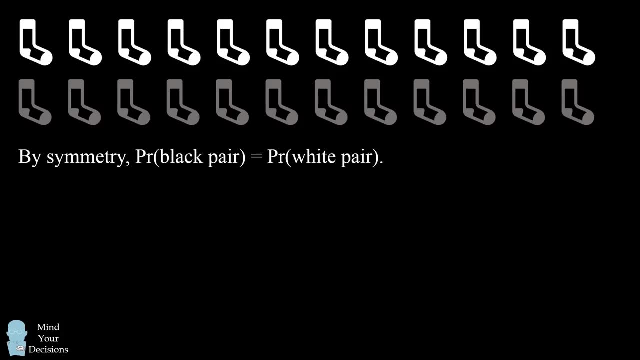 But this tempting answer is wrong. The probability of making a pair is actually slightly less than 50%. Let's calculate and figure out why There are 12 white socks and 12 black socks. By symmetry, the probability of picking a black pair of socks equals the probability of picking a white pair of socks. 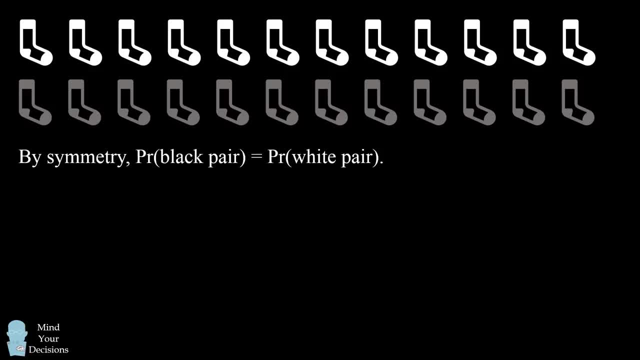 So let's calculate the probability of picking a black pair of socks. There is a 12 over 24 chance. the first sock is black. This is because there are 12 black socks out of 24 socks. 12 over 24 simplifies to be 1 half. 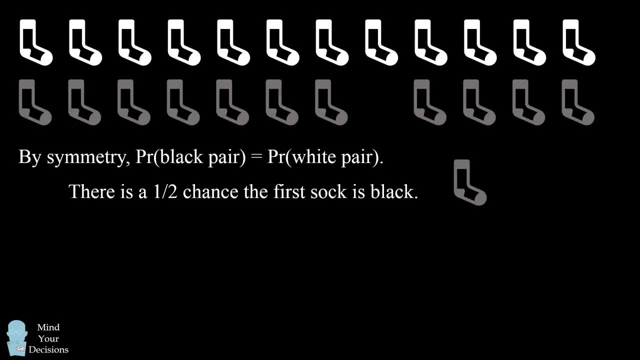 Now what's the chance of picking a black sock on the second draw? For the second sock, the chance will be 11 out of 23, because there are 11 black socks remaining out of a total of 23 socks remaining. The asymmetry is because we are sampling without. 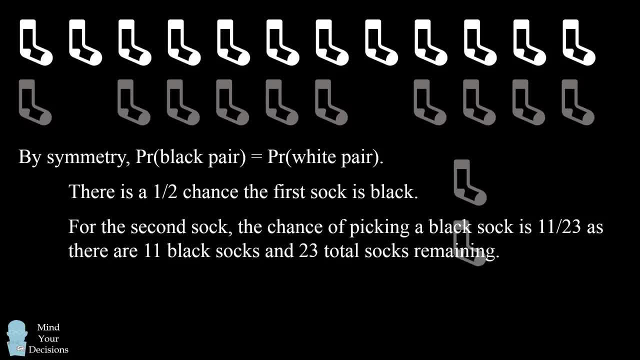 replacement. So what does this all mean? It means the probability of picking a black pair is 1 half times 11 over 23.. This will also be the probability of picking a white pair by symmetry. So we can put this all together to get the odds of picking a pair of matching socks. 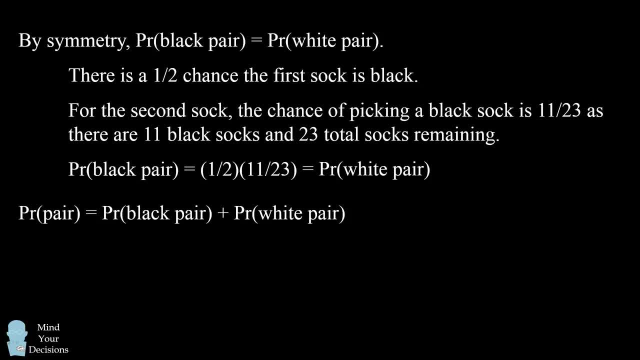 The probability of picking a matching pair will equal the probability of picking a black pair plus the probability of picking a white pair. Each of these is equal to 1 half times 11 over 23, and therefore the probability of picking a pair of matching socks will be 11 over 23,, which is approximately.